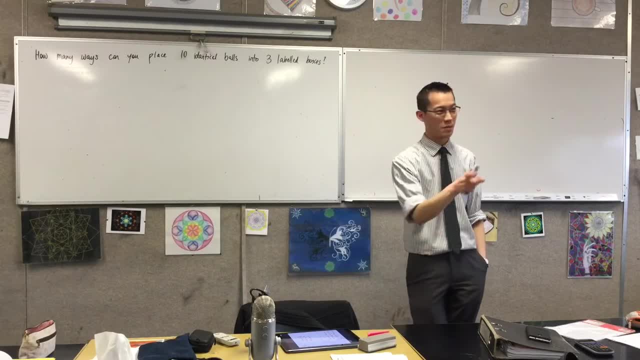 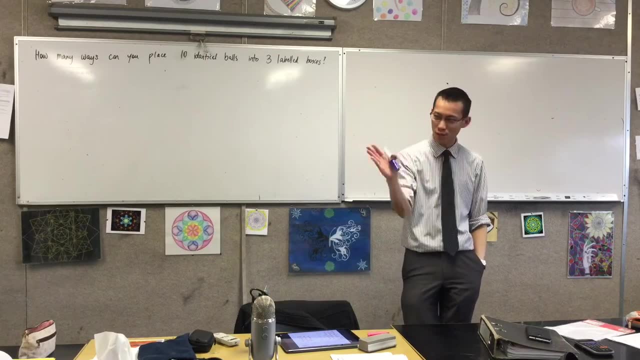 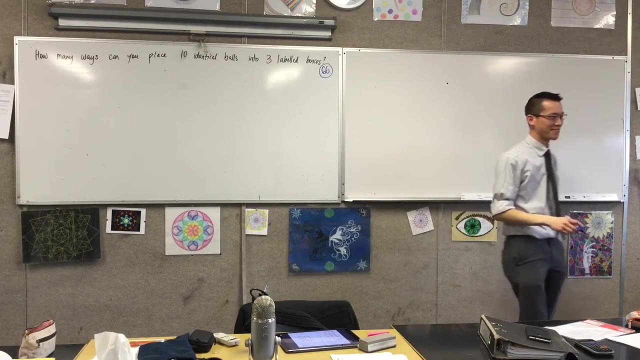 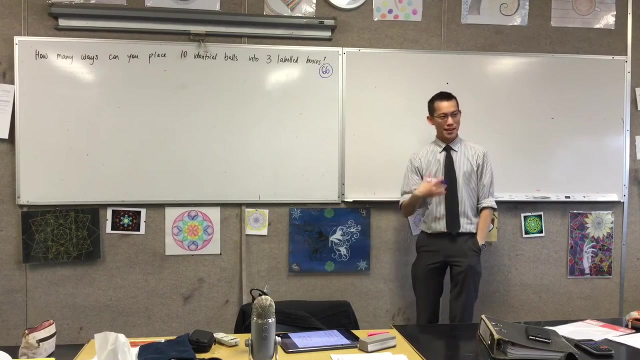 You're so committed to it that you're like no, the answer is wrong. If you get told something different, then you don't really know if your answer is the answer right. So that means that doesn't mean a bad thing, You got the right number, but it means you still got a way to go. Okay, so the answer is 66. So congratulations if you got 66.. However, it's worth pointing out, I can come up with the number 66 by stringing together a random series of like: add this and multiply that, Aha 66. 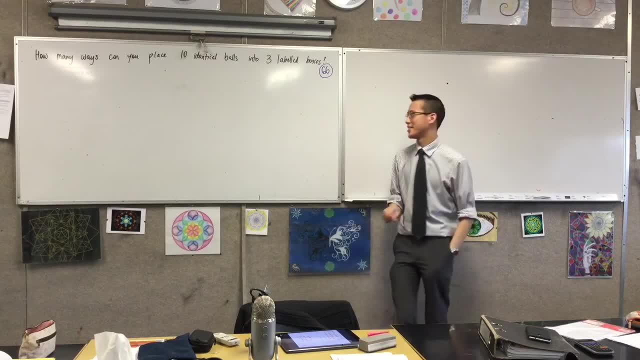 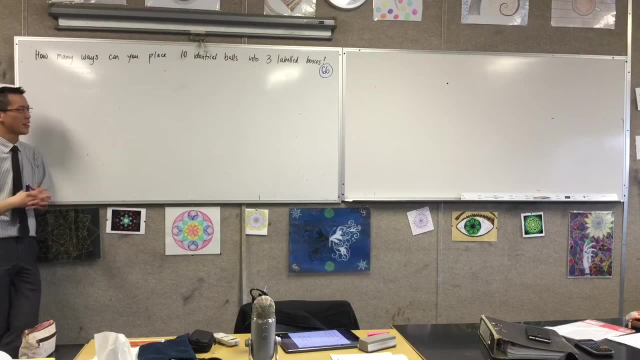 And you might not be able to demonstrate why it is 66.. Okay, so my three clues- my three clues started with, come up with a simpler version of this problem. Okay, remember I said to you, if you have a simple problem, you can list things out. then list them out. One of the wonderful things about this is that it's sort of self evident. You're like, well, there, they are right. Like I've got all the ways, So you don't need to necessarily worry about like, did I miss a type Or did I miss a number? 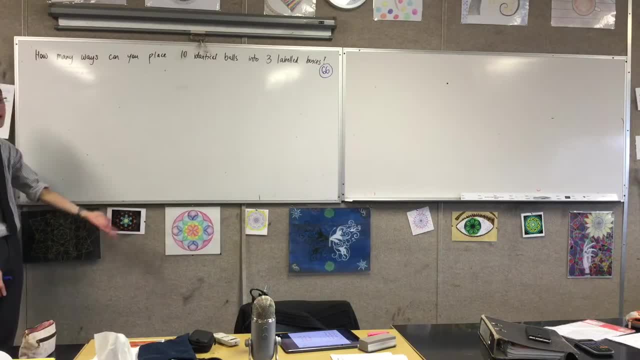 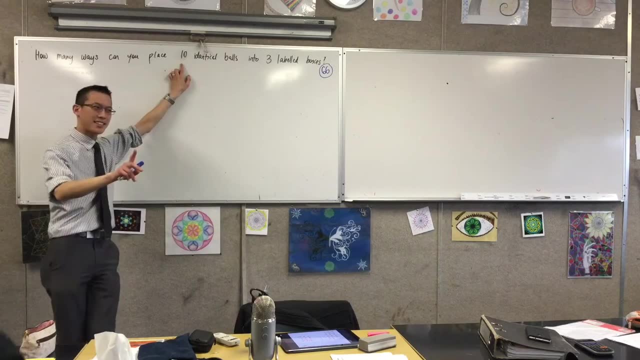 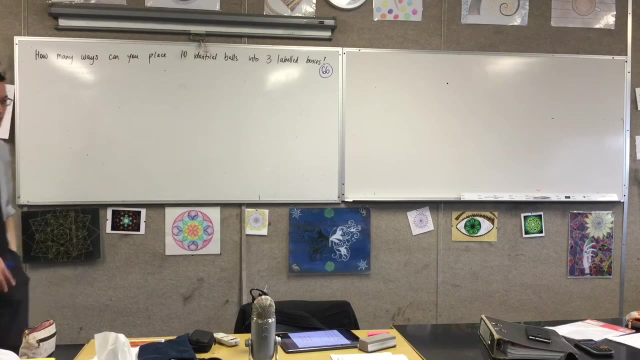 Or did I look at it the wrong way? It's like I've got, I've written down all the ways. Now you can't- despite- Brendan, you know, trying, you can't write down all the ways, At least even with this, like that's actually physically possible, But most people will not be systematic enough to actually get all 66 and not miss any and make sure they've got all of them. I had a Pokemon image that came to my head, but not going to say it Okay. so what you should do instead is: let's boil the question down. Let's imagine if we had something. 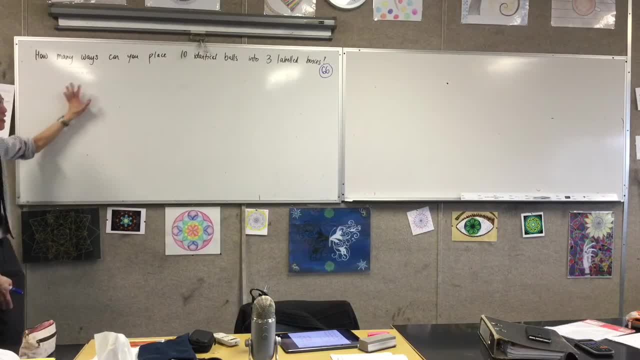 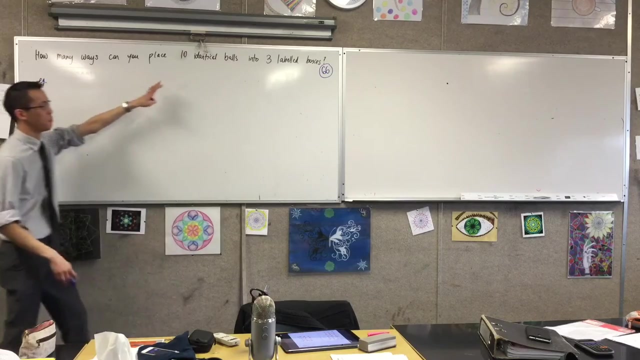 simpler right, Because then I can actually can list them And then I can try and use principles there to convince myself of the answer. Okay, so what would be a nicer, smaller number of identical balls to put into three label boxes? Now, to keep things interesting- maybe you want to do this with me. I think probably a reasonable number that's still going to have enough. in common with the question that what principles I gained out of it will help me. I'm going to go with three, So 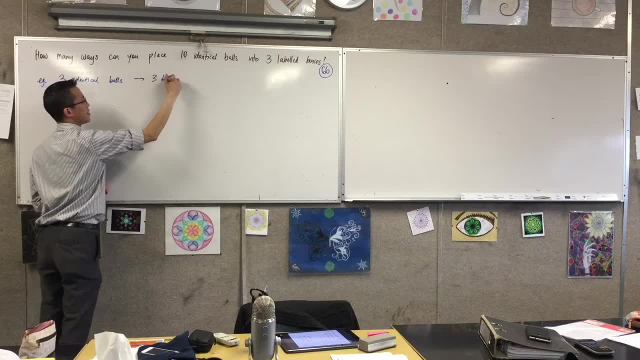 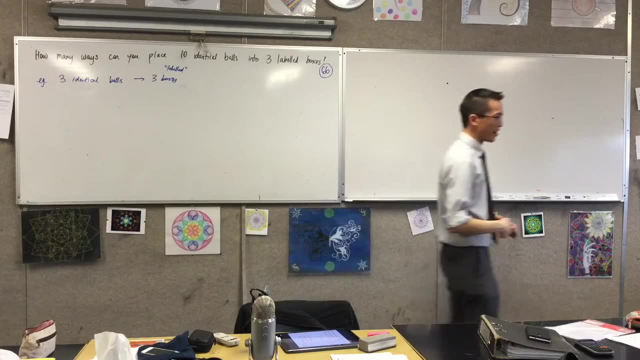 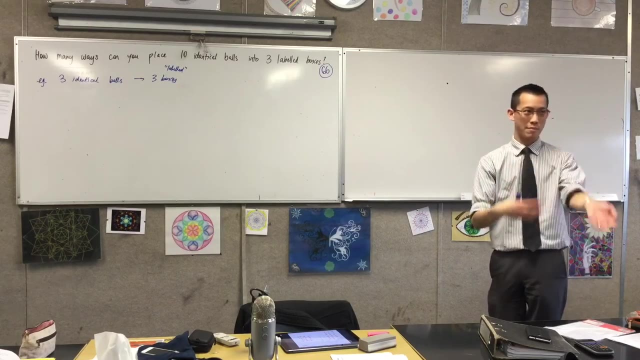 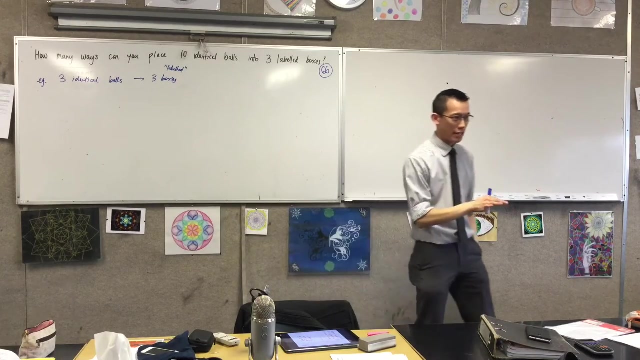 this is a question Whoops. I should say labeled. by the way, The place where I got this question from didn't say labeled, which actually changes the question a little bit. This means I can tell the boxes apart, right, There's like box one, box two, box three, or red box, green box, blue box. Okay, so these can be distinguished, But these cannot Now with three, with three. there are 10 ways, There are exactly 10 ways, And you can help me work out what they are. 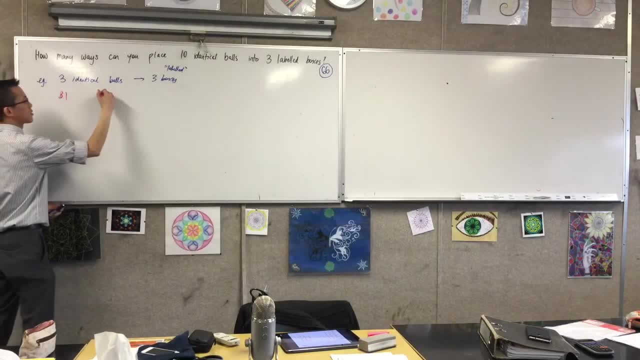 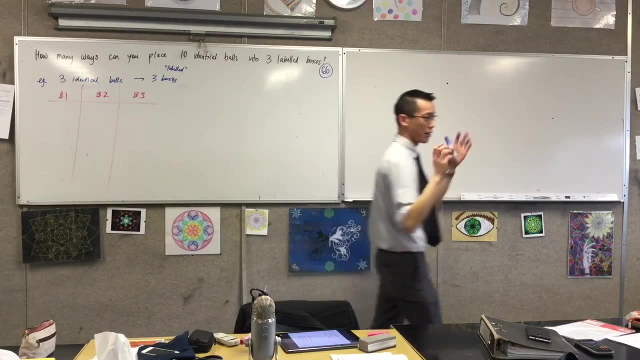 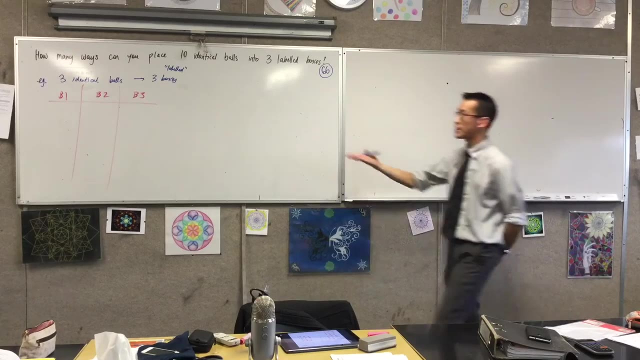 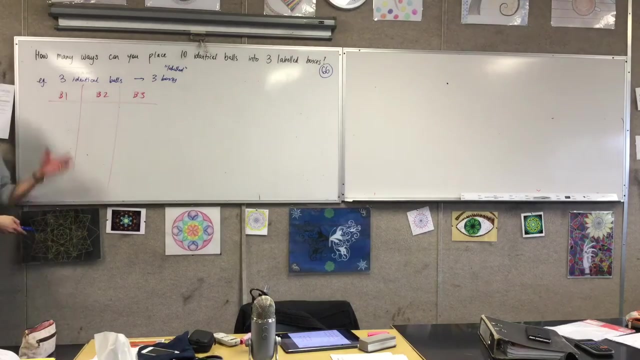 So you can ask questions. Let's imagine you've got box one, box two, box three. We already had this discussion, but just for the sake of the record, can you have all of your three identical balls in one of the boxes? Of course you can, because you're still placing them into boxes. You just happen to leave some of them empty. Okay, so try and think about this in a logical way. What might be a way that you start start listing out the ways you can place, like, how many in here, how many? 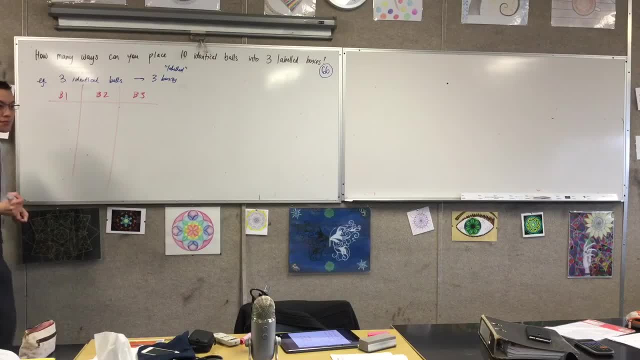 many here? how many here? what's a nice logical way? okay, yeah, cool. I think that's about as simple as I can get. right, take them all there. they are okay. but as soon as you write that down, if you're thinking about it systematically, there are other ways that are very similar to this, but different enough. 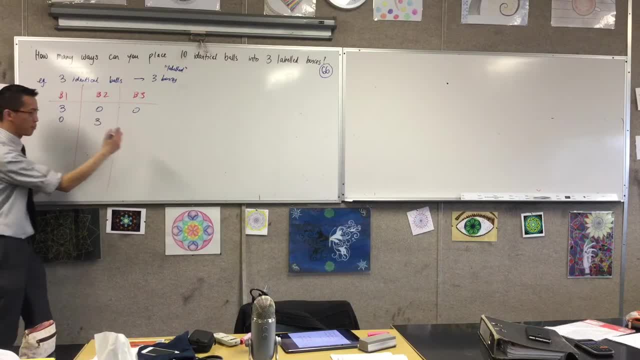 right. for example, let's take the same group and put them all in there, or take the same group and put them all in there. good, okay, I guess a way I could say this is: this is all the ways of arranging by using one of the boxes. does that make? 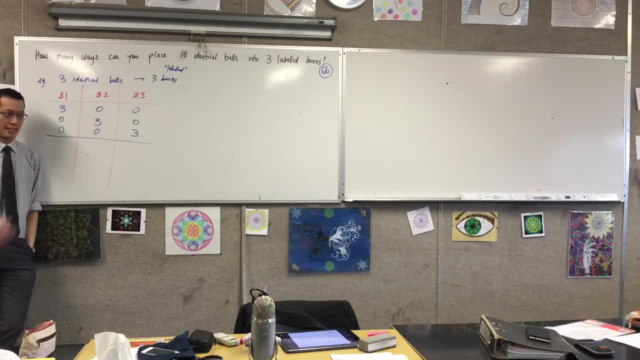 sense. okay, now I'm trying to stay logical right and list them out in a systematic way. if this is the ways of doing it- by using one box, how many ways are there if I use two boxes? okay, so if I use two boxes, one of them is gonna. 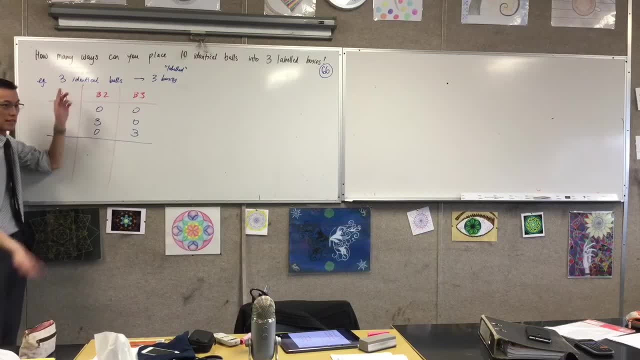 have two, and one's gonna have one right, and then the last one has zero. okay, that's the only ways to do it. so, for example, I could go to one zero, give me another one. now, interesting, I'm gonna go for two zero one, because again, I want to list. 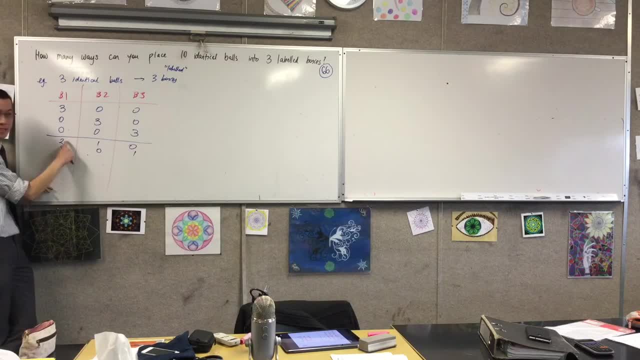 this out in a systematic way so I don't miss anything, right? so I'm gonna keep these the same and then swap these right, and then I'm gonna have another two like this: right one, zero, zero one. you see how I'm trying to do this in a systematic. 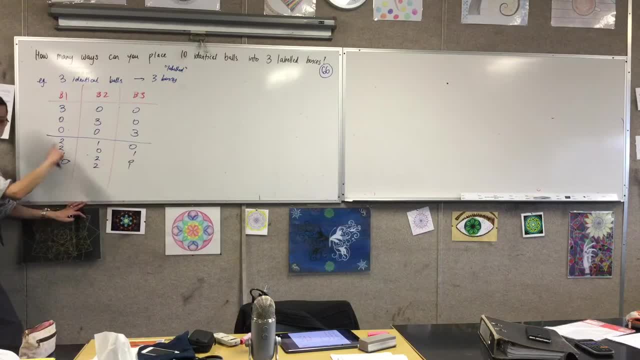 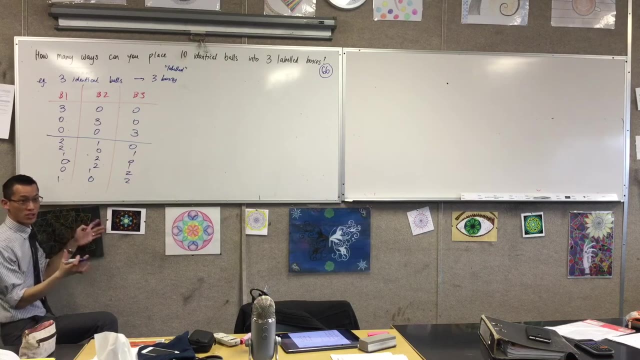 way, so I don't miss anything. I'm still in the scheme of using two, two boxes. so the last one, grab a seat. it's going to be two, two zero, one, one, zero, happy. are there any other ways that I can use just two boxes, just two? 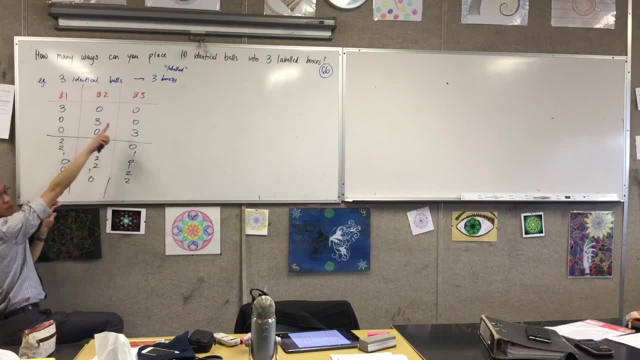 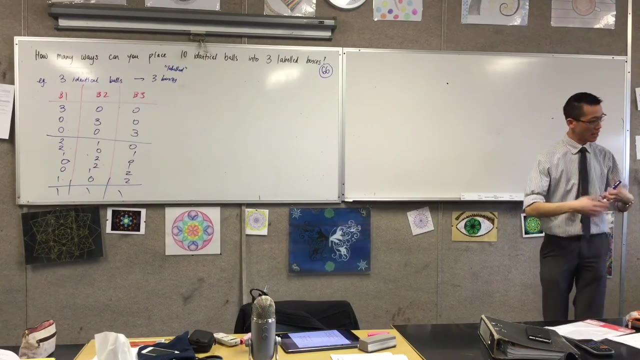 boxes. that's it, right, that's it. so I've got one box used, two boxes used. how many ways can I use all the boxes? there's only one way, right? okay, so there's ten options. that's it. and, like I said, the wonderful thing about a list, like I think. 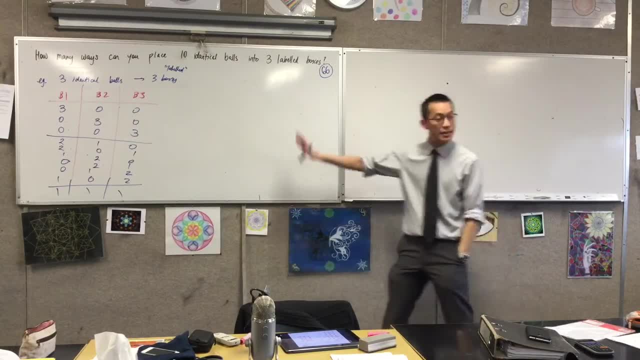 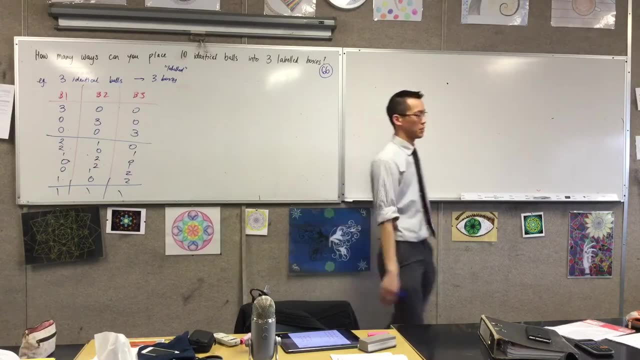 we sort of look down on lists. right, it's like what a pedestrian way to do things, but it's self-evident. there's no other way that you can do this. one box, two boxes, three boxes, all the options. so then comes the challenge of thinking. 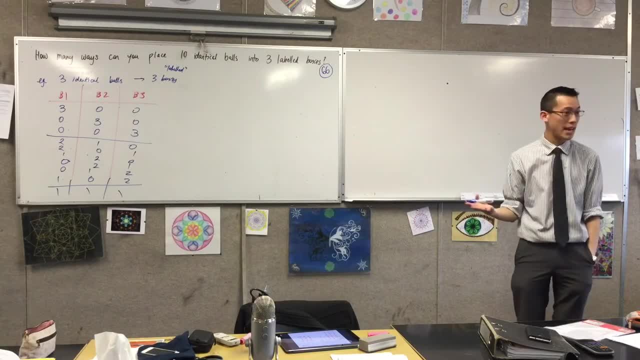 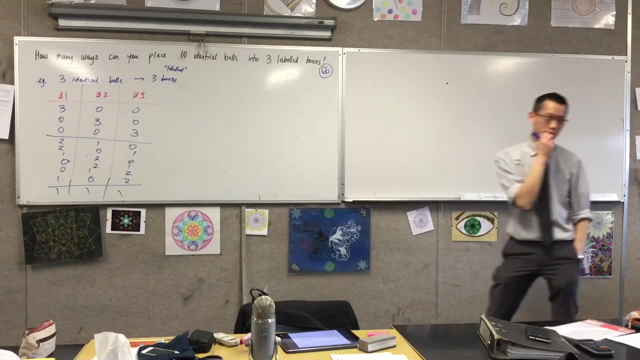 well, how can I come up with the number ten? in what ways can I work out ten? coming through in here right now to try and get at the logic. to try and get at the logic. my second clue, my second and third clues, are actually two halves of the. 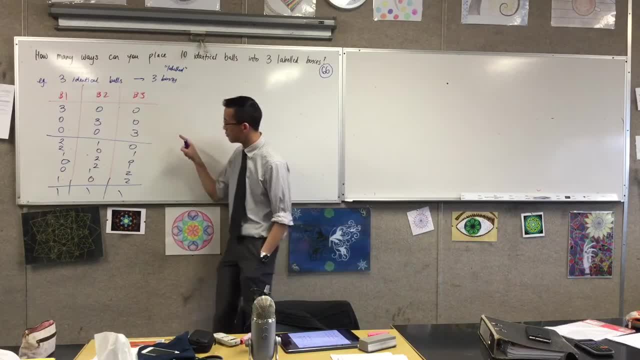 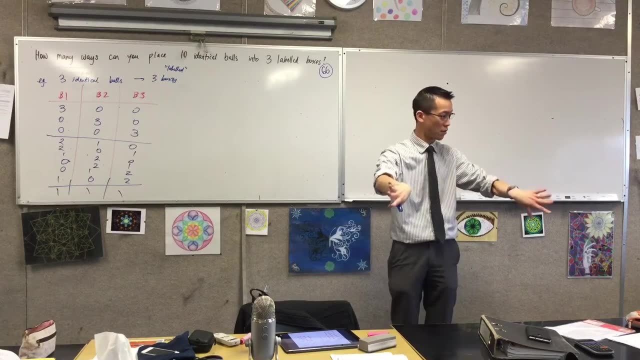 same clue. they would think about this not in terms of putting balls into boxes, but thinking about the balls being already there and ways to separate them into different boxes, right? so here is like, if you can imagine this way, here the balls are movable, right? it's like, oh, where? 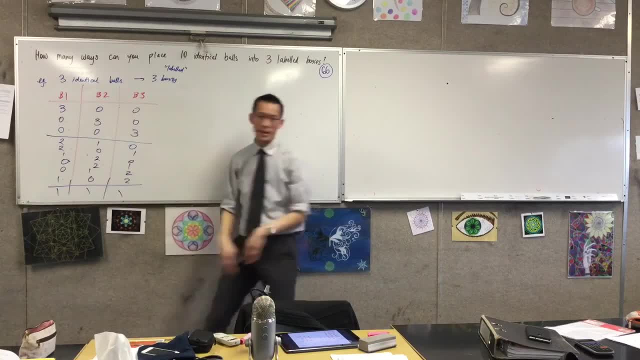 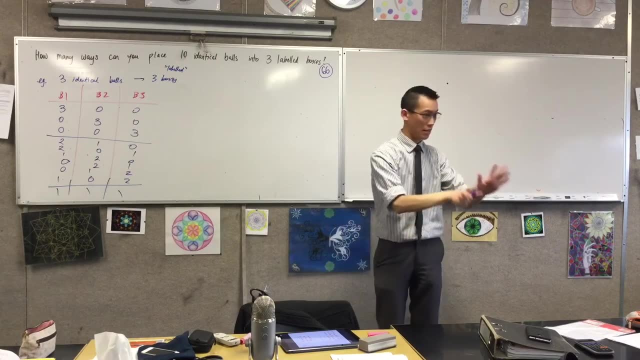 should I place them and these things are just fixed. okay, my second scheme of thinking about this is: well, what if the balls are fixed and I'm trying to designate: these ones go in this box, these ones go in this box, etc. okay, so there's at least two ways of thinking about this. okay, now, Jinsoo, if this: 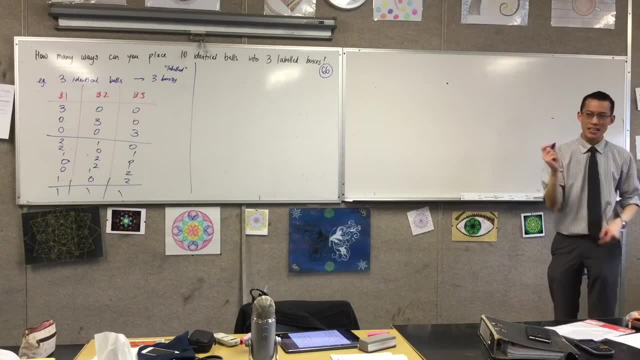 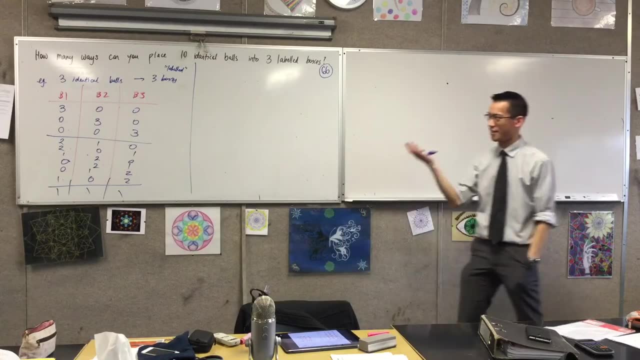 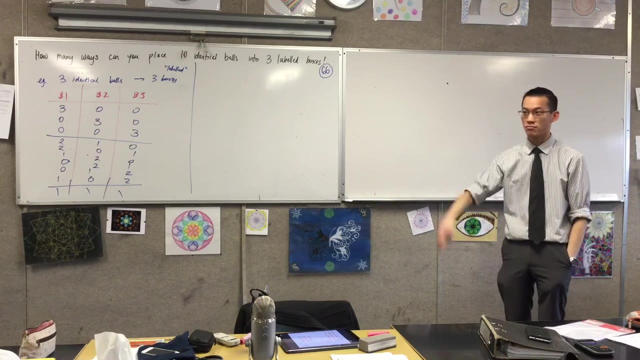 is the first point. I'm gonna pause and ask you to explain the class. how did you, what extra idea did you introduce? because this is just balls and boxes, but you had a whole extra idea that helped you think about this. what was your way of thinking about it? just just explain what you did. you had more than just the 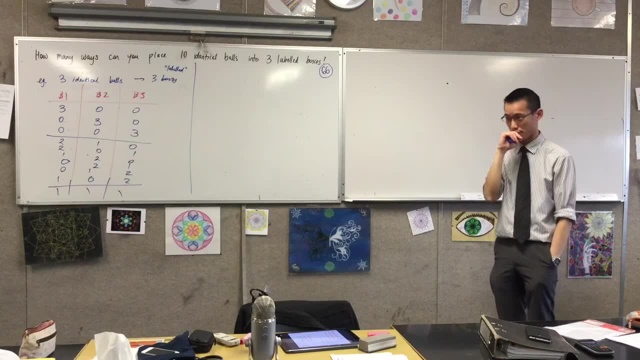 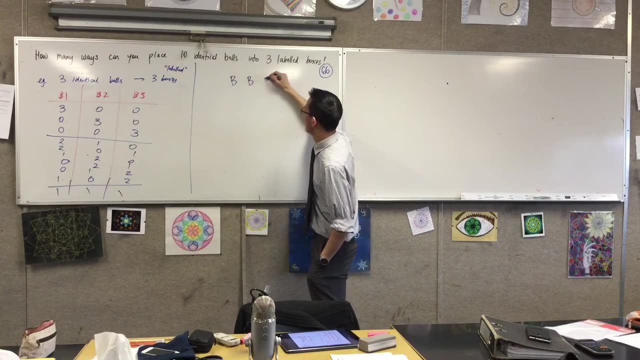 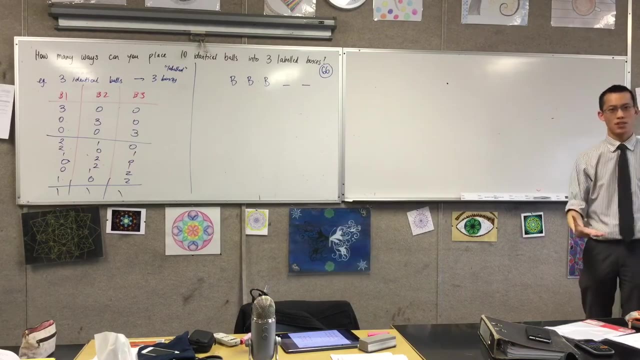 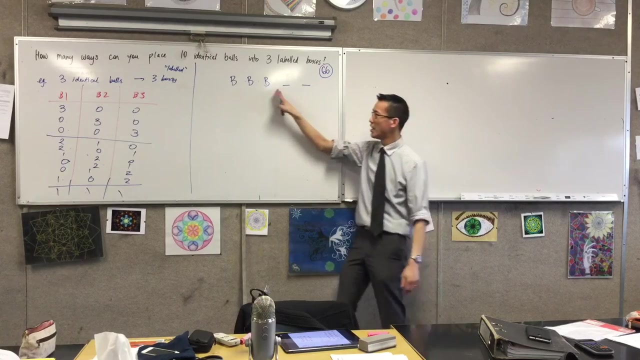 balls to place. you had something else that you placed. remember that. yeah, okay, okay. so this is a new way of framing the question. right, there's nothing that gaps in the question, but we can introduce these guys as our mechanism for saying: okay, some of these will be in the first box, some of these will be in the 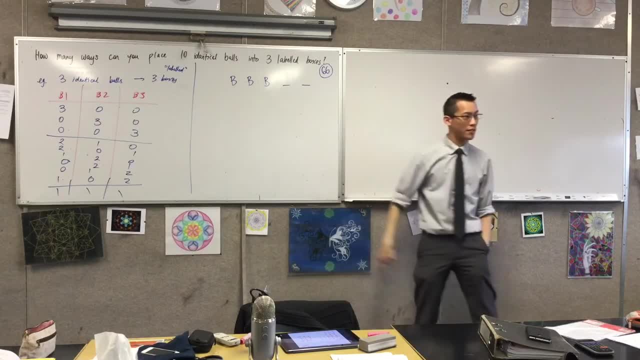 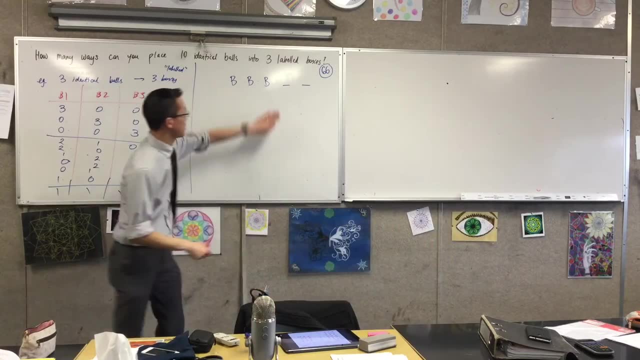 second and some will be in the third. okay, for instance, this is one of the arrangements. this is one of the arrangements. in fact, it's the first arrangement. okay, can you imagine? everything to the left and to the right of this gap is the first box right, and then everything in here is the second. 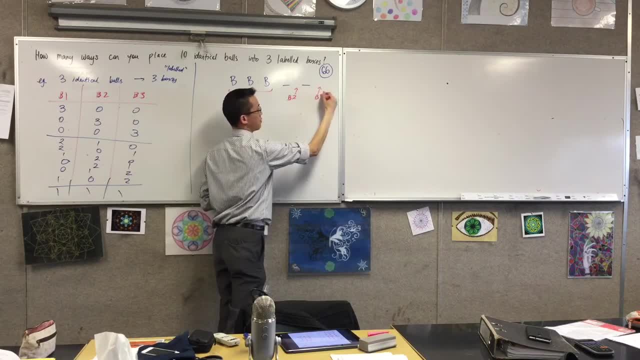 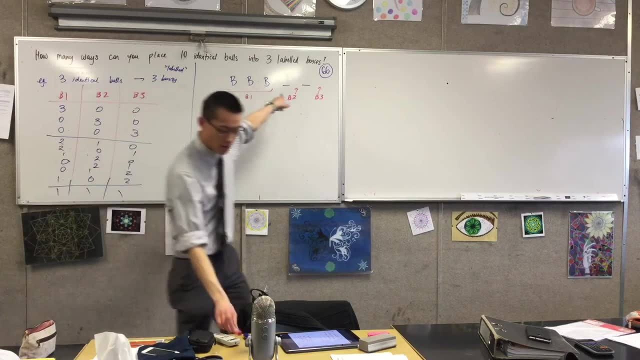 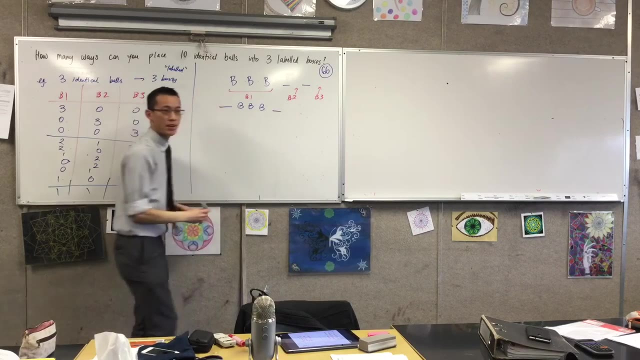 box, right, and then everything over here is the third box. so this is three zero zero. do you see that? how would I do this one? how would I do it? what kind of way would it be? balls and gaps together. yeah, yeah, very good. okay, look, see everything. 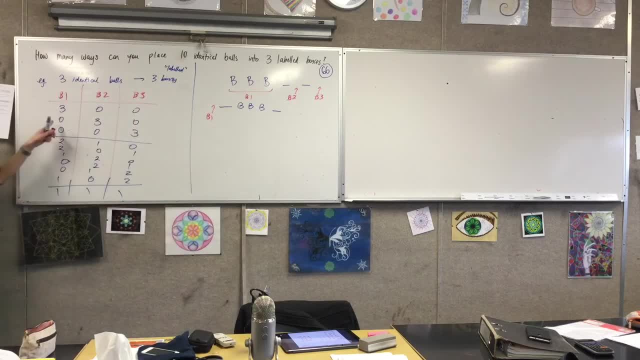 before the first gap, that's what's in box one, which is none of them. then here is box two, and then here is box three, and it's also empty. you see how this works okay, and you can say any of these in this way and it'll work okay. so how? 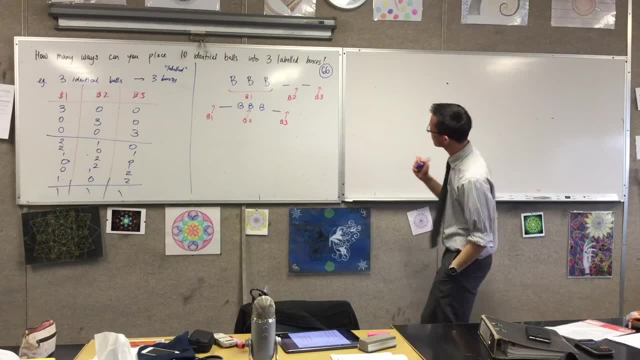 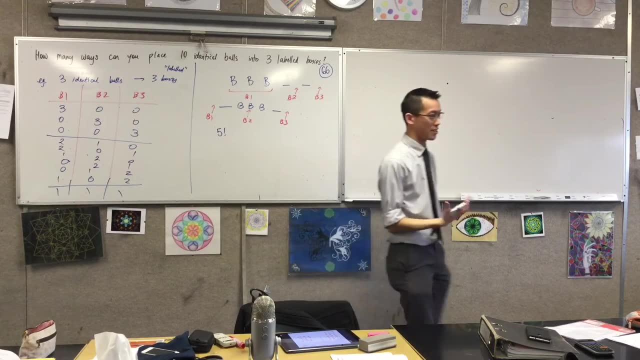 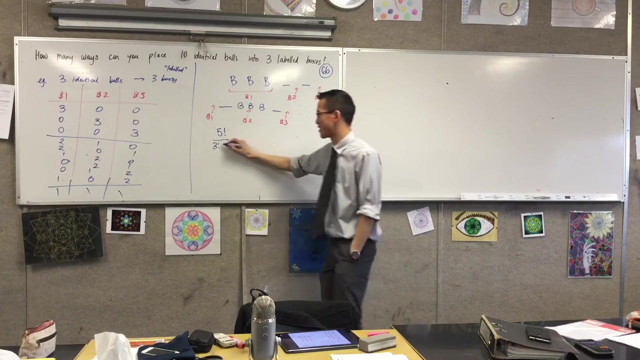 many objects am i arranging? I count one, two, three, four, five objects, right? five objects are, but some of them are identical, right? how many identical things do I have? these balls are all identical, so three factorial. and then the gaps are also identical, right? I can't tell the difference between them, right? so that's. 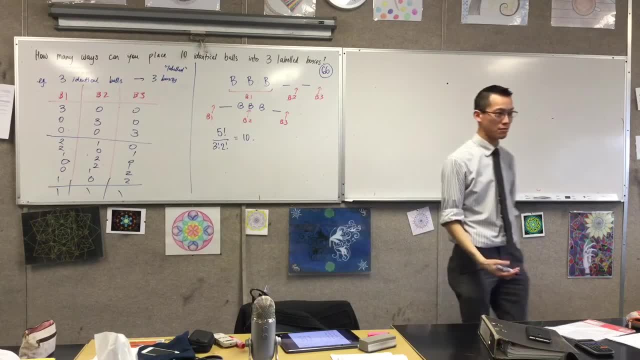 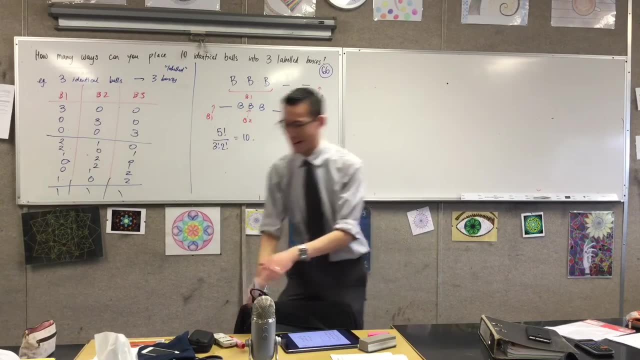 ten, that's ten. yes, okay, now, that's not the only way you can think about it. you can think about- and this is the way that Liz was trying to, but didn't quite get there- you can think about, and I actually um, I don't know if you remember this. 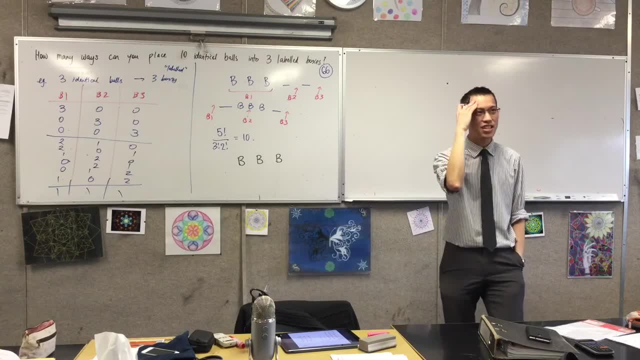 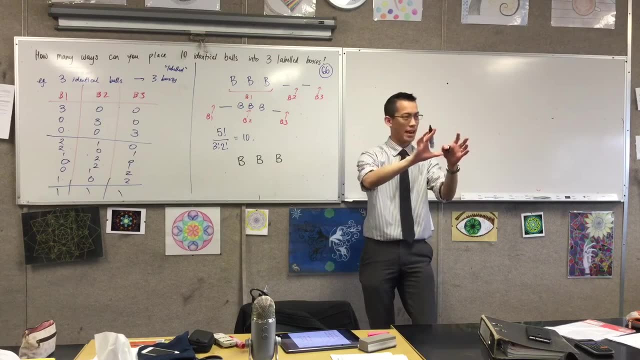 when we did one of those like what was the word? I gave you decisions, I think it was, and you had to think about it. and you had to think about it and you had to say: okay, how many ways can I arrange where the D is to the left of the N? or? 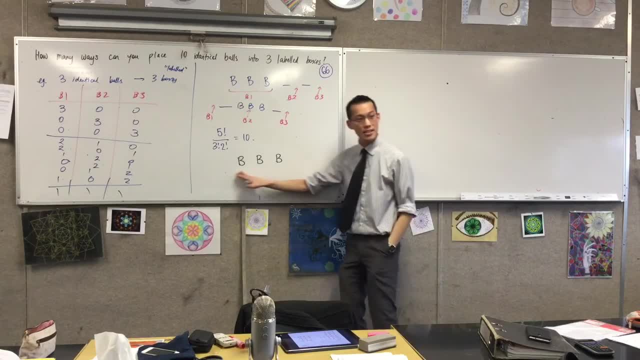 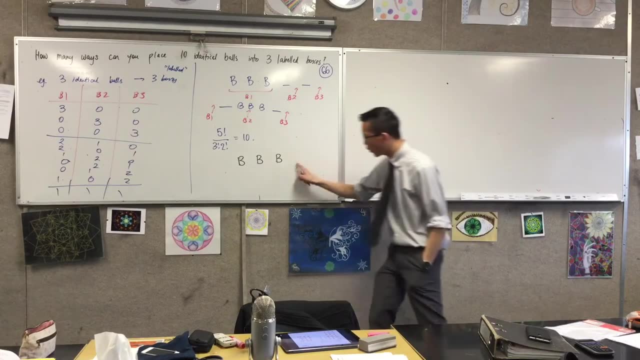 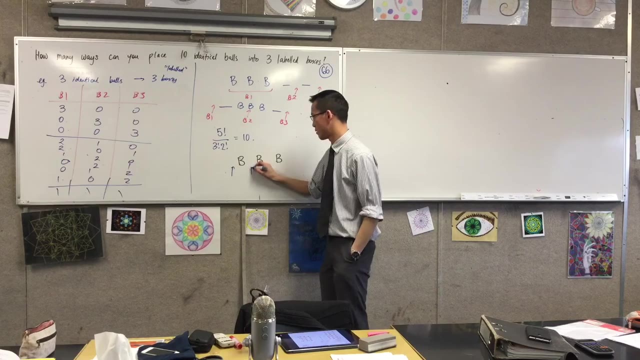 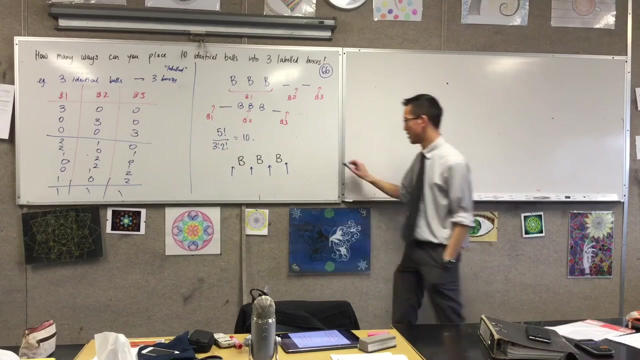 something like that. okay, right, so if I fix these guys in place, right, I can think about arranging the gaps. now, how many places are there where I can put a gap in here? how many ways I count? four, one, two, three, four, right, but there's a secret one. there's a secret one. how many gaps do I have to? 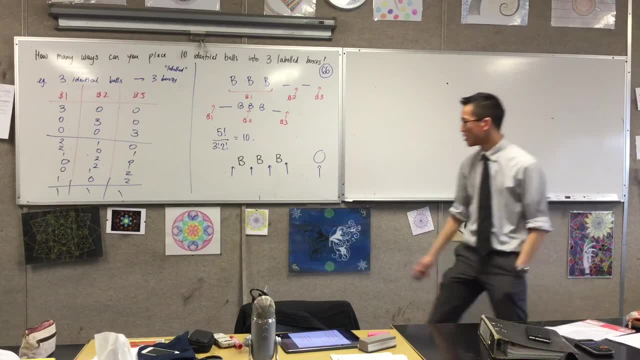 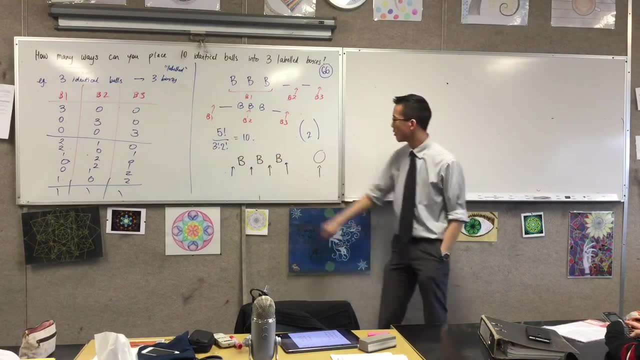 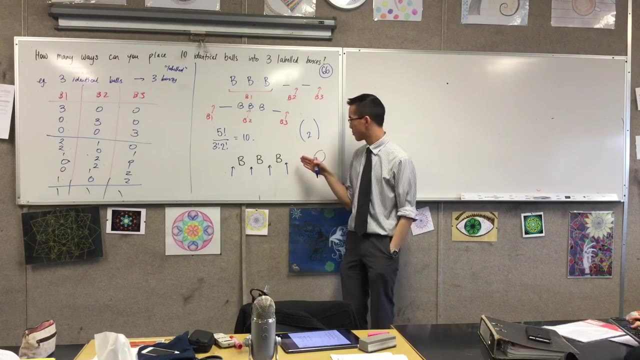 place again how many gaps. I have two gaps to place, so this is going to be something choose two, right, something choose two. oh, by the way, yeah, we already established this is ten. right, something choose two. now I'm saying that, okay, you can put it here, here, here or here, right, but actually, once you place one of the 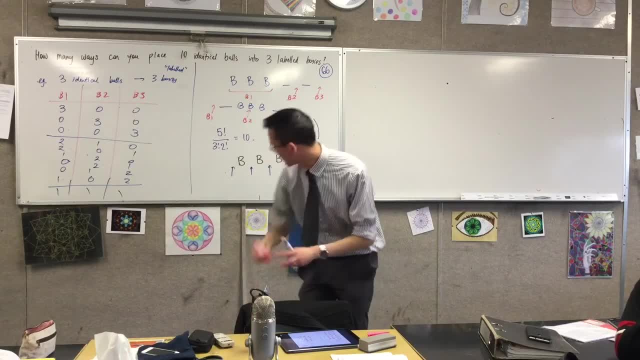 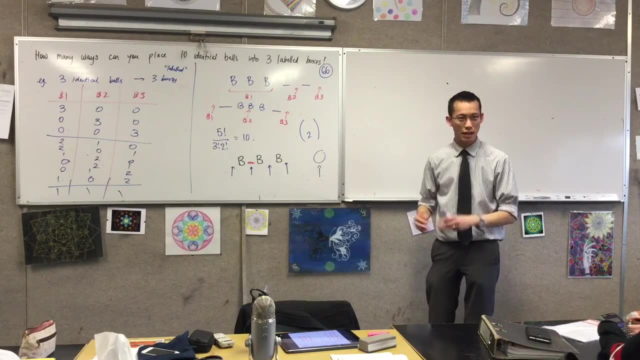 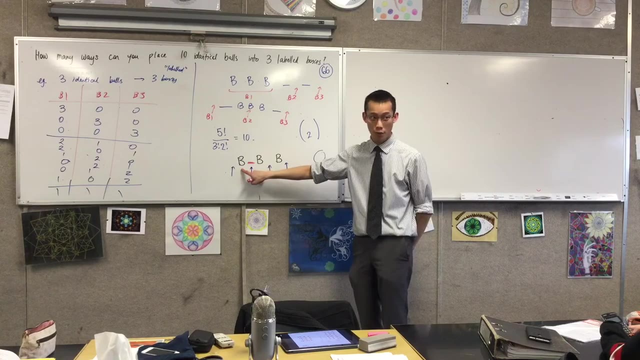 gaps. okay, like, say, I place a gap here, let's put it here, let's place a gap there. okay, at the moment, what does this configuration look like? where are, where are all of the um, the balls in this current configuration? this one is in the first box and these are in the second box. right? what if I didn't want to place? 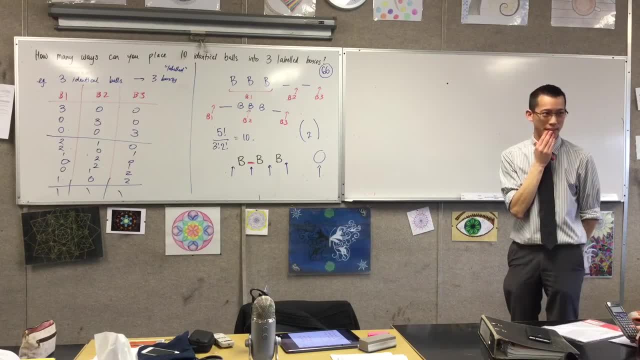 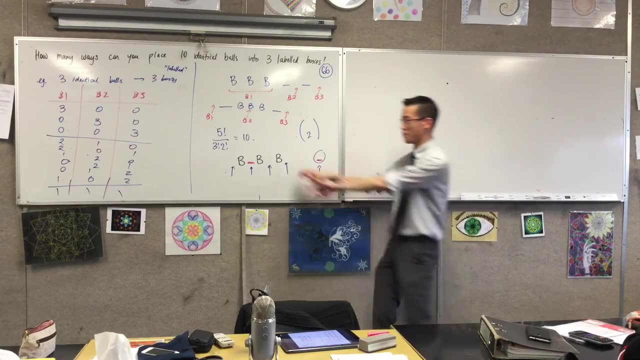 any in the third box? right, where would I put it? the answer is: I wouldn't use that gap. that gap I don't need, right? I've already separated them into two groups. okay, so I've got the first group, second group and I don't need to divide them anymore. 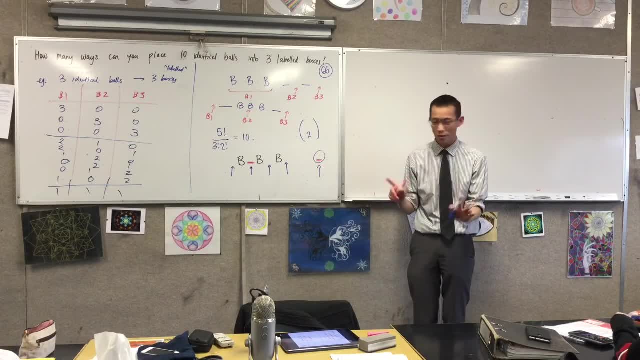 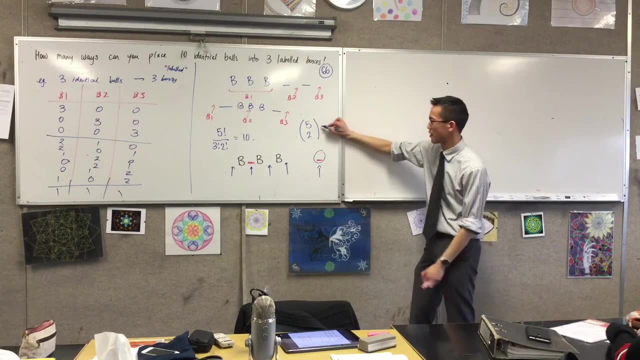 does that make sense? so I've got one, two, three, four, five spots where I can put a gap, and I have to choose two of them and you will find privacy. two is also ten, because that is in fact five C two. okay, but we arrived at this in kind of a. 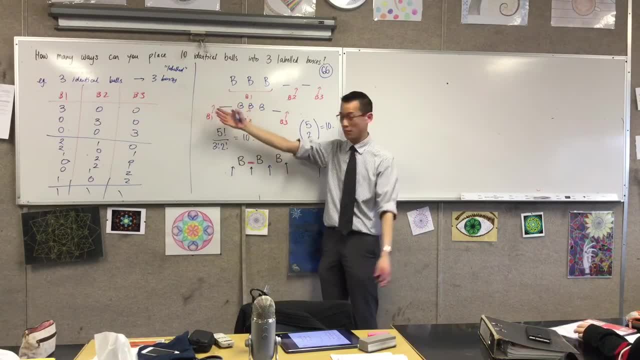 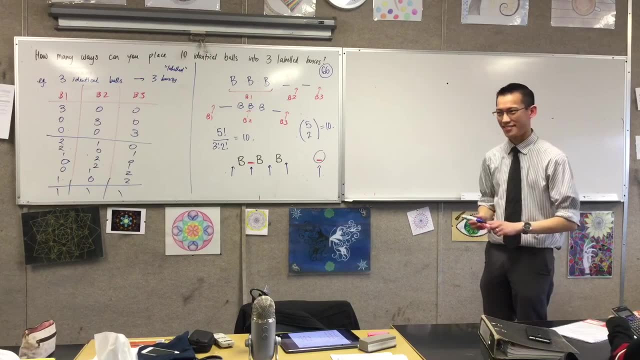 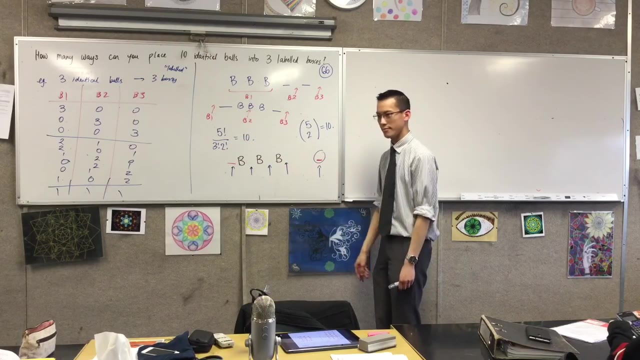 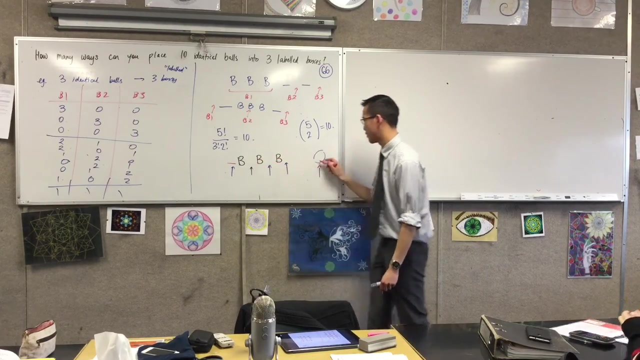 different way. right, we're arranging objects is a permutation, the order matters, right, but then you have these identical things. does that make sense? yeah, at the very front, I can still do that, right? or this is a different arrangement. again, right, so I can use the second gap or I don't have to. I don't have to use. 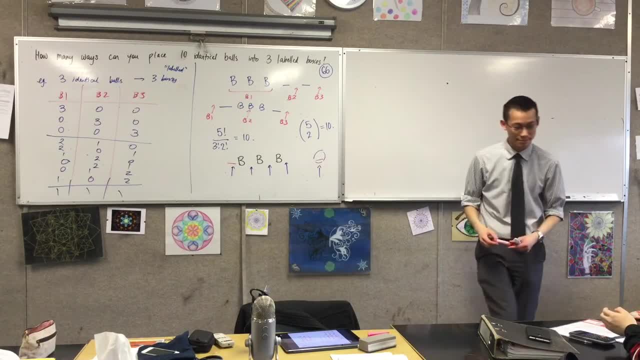 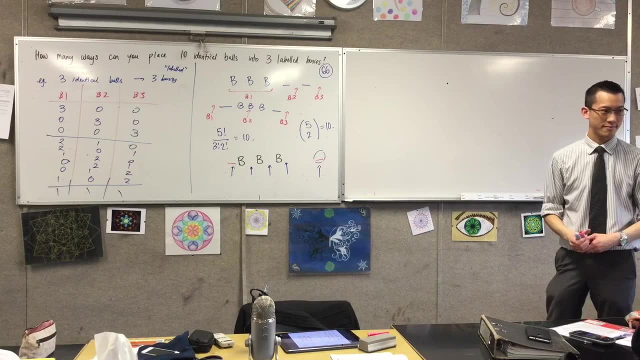 it right? yep, could you think about this like? this is way like. could you think about it as not having a mystery gap, but when you actually face a gap, you can place another gap right next? yes, yes, you can. yes, that's exactly right. you can place another gap right next to it. yes, yes, you can. yes, that's exactly right. 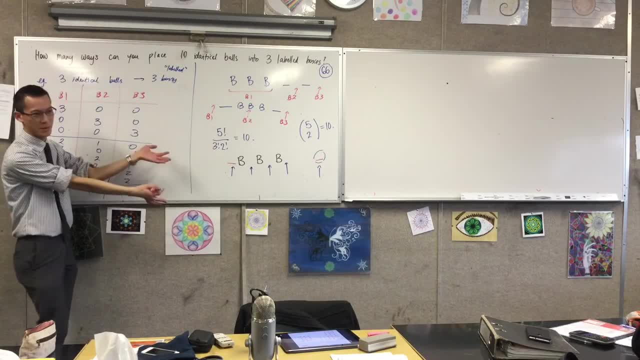 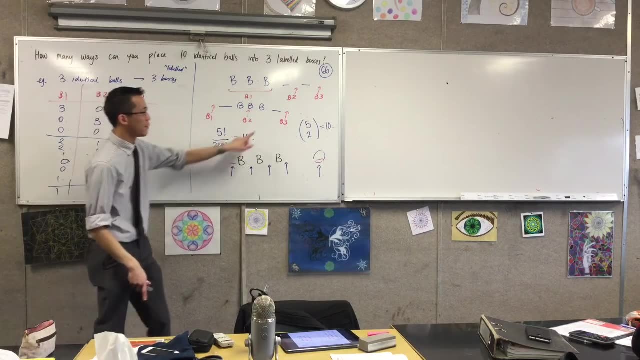 so that's another way of thinking about it. I contemplated using that as my explanation, but then I thought, yeah, I I get confused because then I'm like: okay, I place a gap, and essentially what you're mentioning is like placing two gaps together, right. so it's like: oh, I've made a new position, right, which is right. 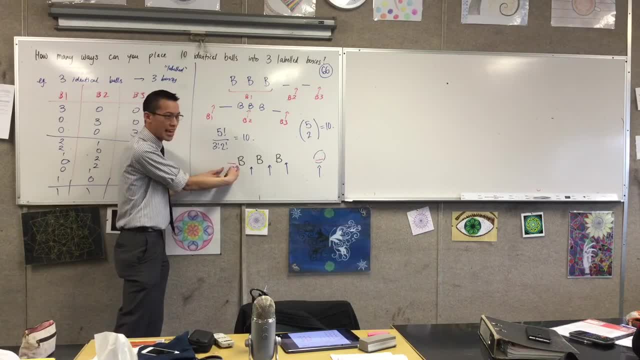 where I am and it doesn't. well, it doesn't need to be two, because I'll put it here or here, it's the same, it has the same effect, right? but I think it's better just to say: don't use that. it has the effect of not dividing anything at. 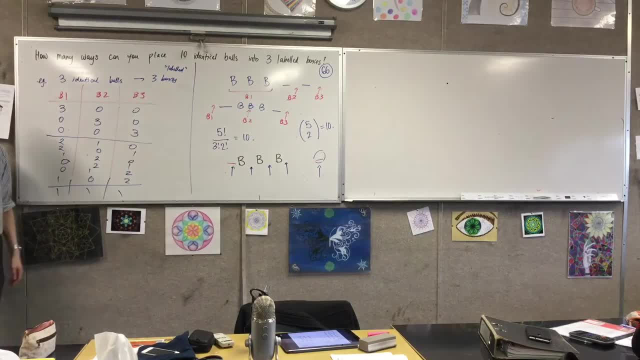 all, so you might as well just put it to one side. okay, so now you're ready to tell me what. the answer to the original question is right, because you've understood the principle in a manageable way. what's different? yeah, yeah, from three identical balls. I added two gaps to that and that's what made it 5 C 2, not 3 C 2. 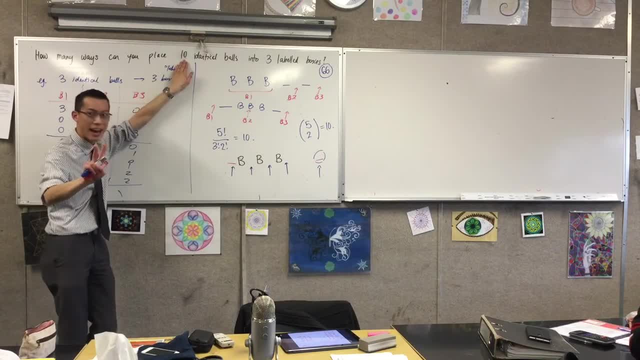 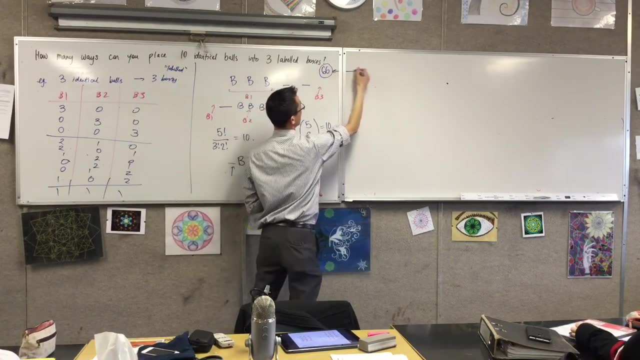 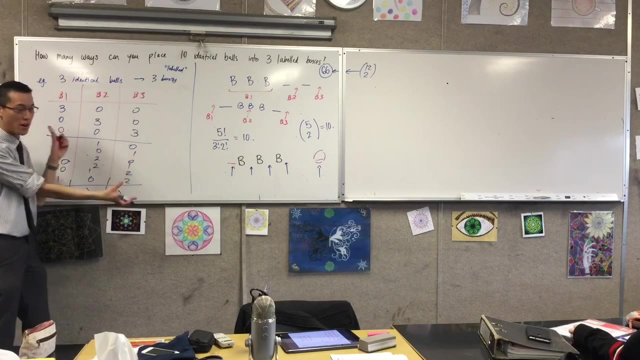 right, but if I have 10 balls and I still have two gaps, then it's going to be not 5 C 2 but 12 C 2, which I think you'll find is 66, and one of the lovely things about this, about having understood the way it works, is that now I can say: all right, what if you? 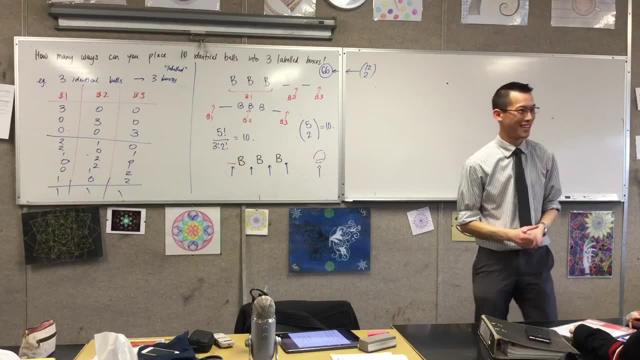 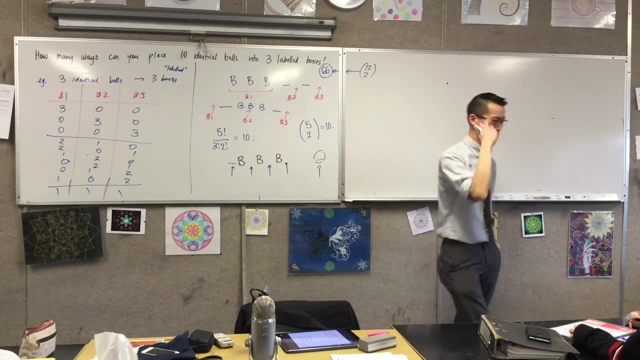 wanted to place them into I don't know 10 boxes. right, that wouldn't be any more difficult for you now that you understand what's going on underneath, whereas if you want to try and go with cases, you're going to be sitting there for a very, very long time. okay, please don't underestimate a lot of people.